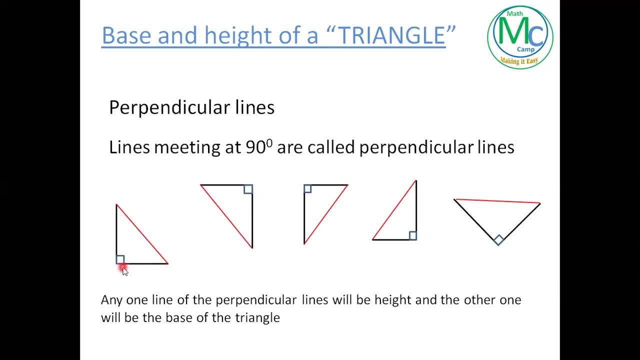 one of the main problems with this triangle is that there is a lot of vertical line You have One of the line, or perpendicular line, will work as height and the other one will work as base. It's totally up to you that which side you want to take as height and which side you 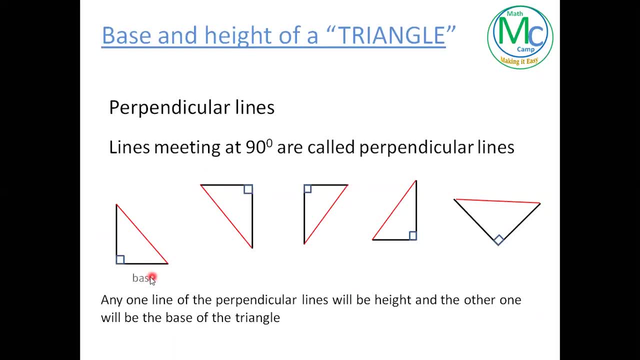 have to take as base. For example, if I take this side as base, then the perpendicular line of this line, which is this, it will be height. Or if you want to change this side as base, to base this perpendicular side for this. 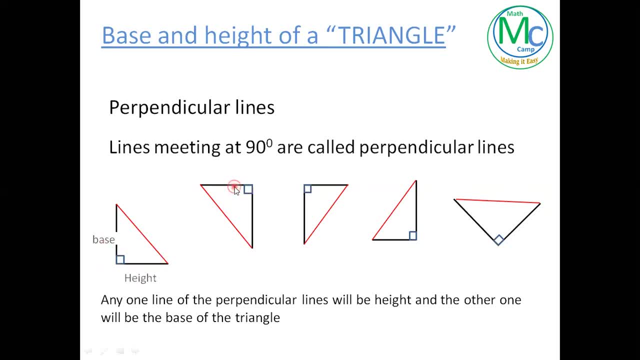 line will be height. So, likewise, if I'm taking this side as base, the perpendicular line to this line, which is this, it will be height For this if this one is height. so this is going to be base for this. 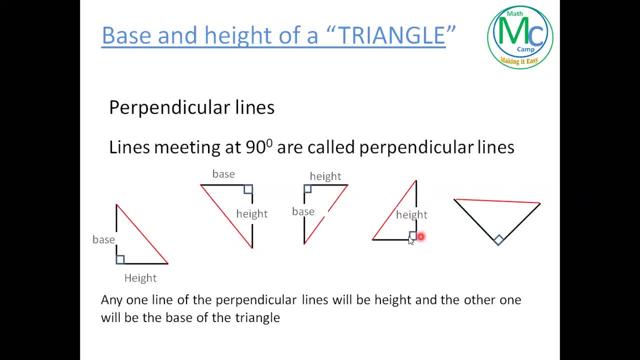 If this one is height, then perpendicular line to this line, which is this: this will be base. and the last triangle: if this one is height, then perpendicular line to this line is this: this will be base. So to find out, 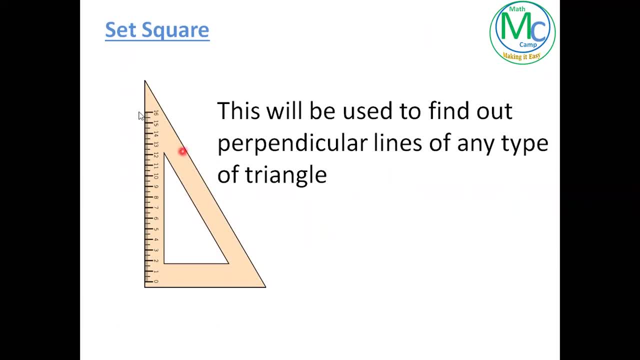 The perpendicular lines. I'm going to use set square. So these two lines of set square are meeting each other at 90 degree angle. So one of the line will be work as base and the one of the line will be work as height. 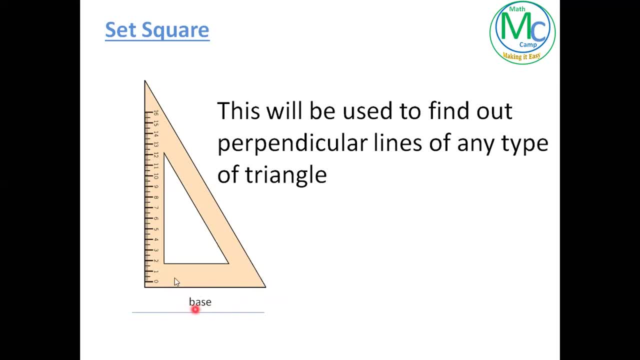 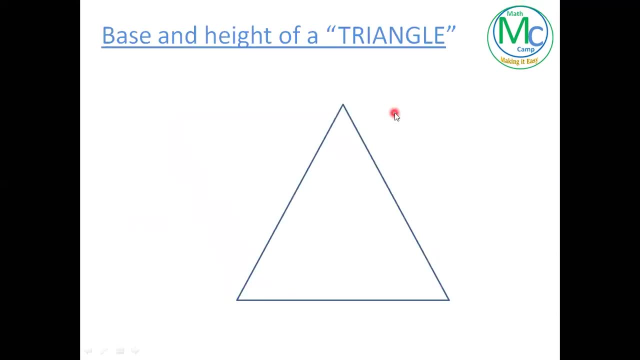 So I'm going to take this side of set square as base and this side of set square as height. So now I'm going to find out height for this triangle and the base of triangle is here. So once we have a base, so I would place my set square like this: the that, the base. 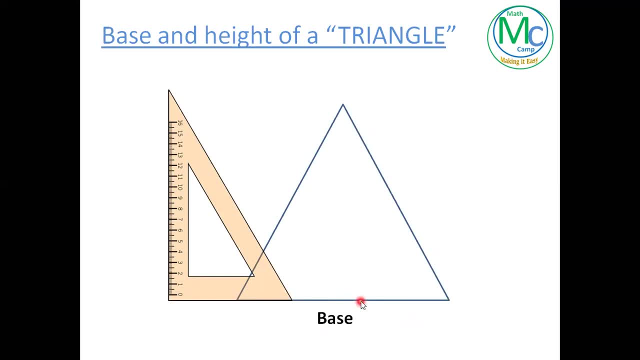 of set square should overlap the base of the triangle. So after that I will slide this set square over this triangle and I will keep an eye on this height of set square. Once this side touch any of the vertex of this triangle, then I will stop sliding. 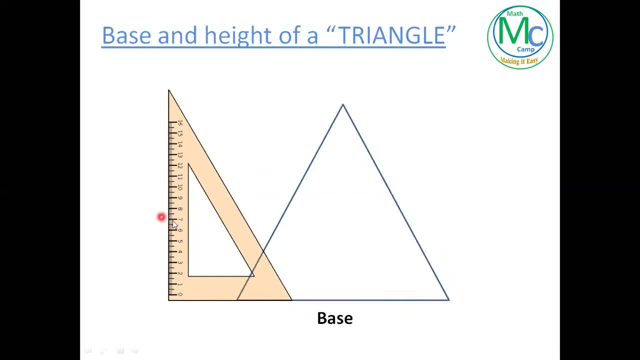 All right, The main purpose is you have to slide this set square and you'll stop once this height of the set square touch the vertex of this triangle, any vertex. So let's see. So I'm sliding this one and I will stop here. 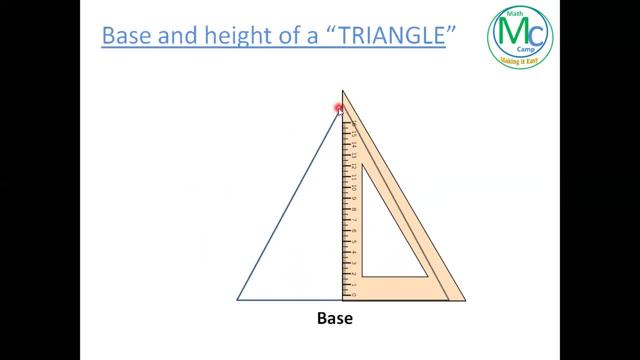 Why? Because this height has touched this vertex, So you can look again. So I will start sliding and I will stop when it will touch here. All right, After that I will just draw this line. So this is going to be height. 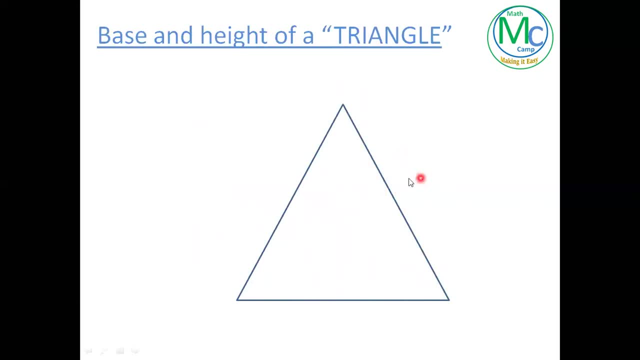 So height for this base is this. Now, what if I change my base? Now, base is this. So what I'm going to do? I'm going to place my set square according to the base. So base of set square should be over the base of triangle. 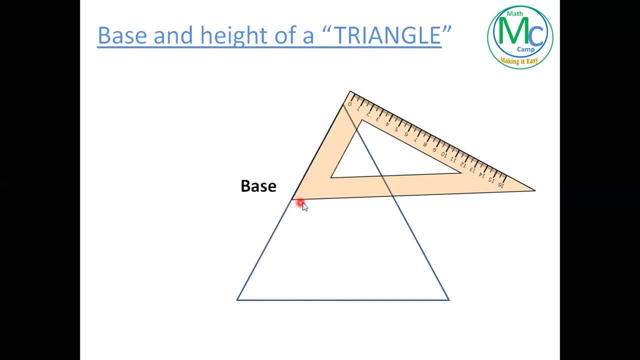 Okay, Okay, Okay. So again, I will start sliding this set square and I will keep an eye on this point once it will touch the vertex. So there we have this vertex, this and this. Once this height of set square touch any of this vertex, I will stop. 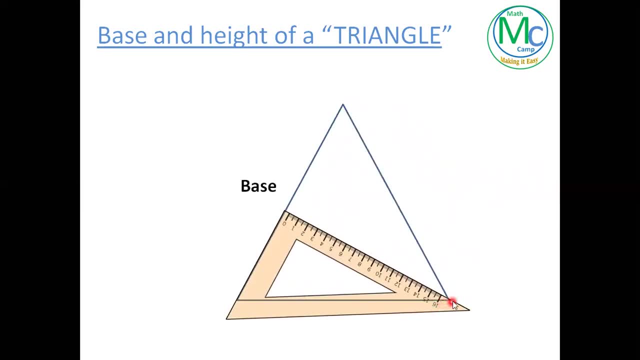 Now look here, So I'll slide, slide, slide and stop here. So this has been touched, this vertex, And then again, using my pencil, I will draw. Okay, Add this. So the height for this base is this. Now, if I change base of this triangle for this one, so I will use same set square and 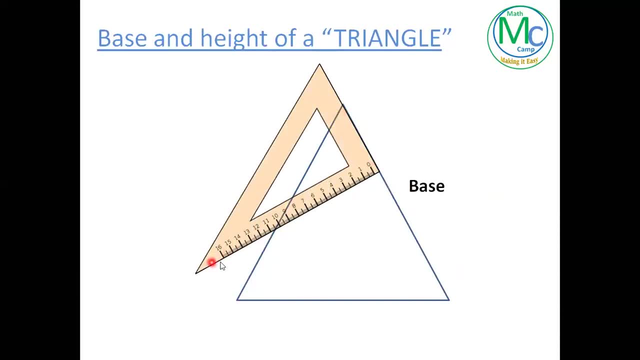 I will place according to the base. Now again, I will. I will start sliding this set square and I will have an eye on this side Once it will touch. I'm sure that you can guess now that when I slide this one over this. so this is going. 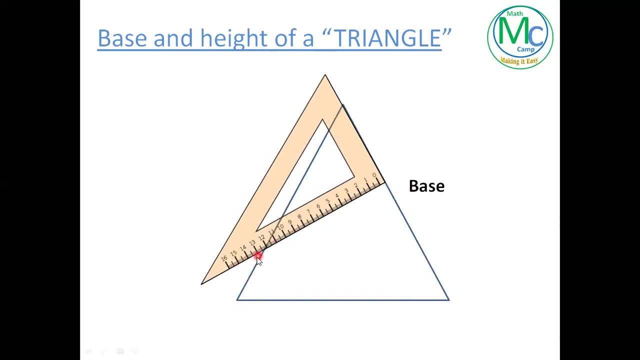 to touch this vertex, this height, Okay, So here, stop, Again. I will draw the line. So the height for this base is this: Now it's your turn, So there's a triangle and this is the base. So you are going to pause this. 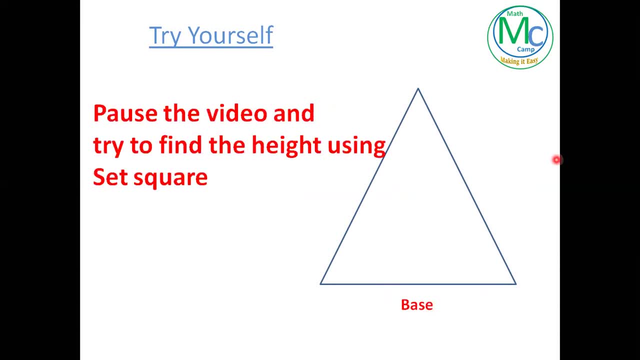 video: find out height for this base. Once you have your answer, you can resume this video. All right, So I'm going to show how to find out, how to find out the height of this triangle. So, again, I will place my set square according to the base. So the base. 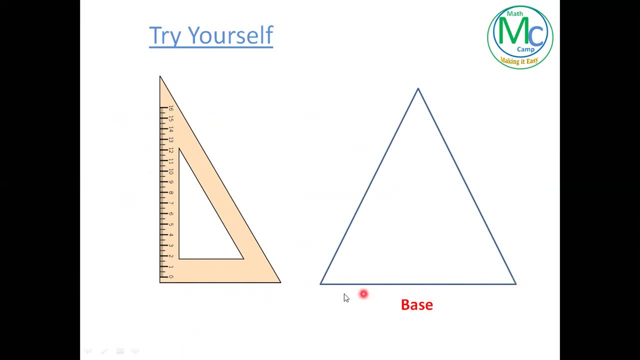 of the set square should slide over the base of the triangle. So the height for this triangle is this for this base, for this specific base, Question number two. try this one now. All right, now check your answer Again. base of set square. 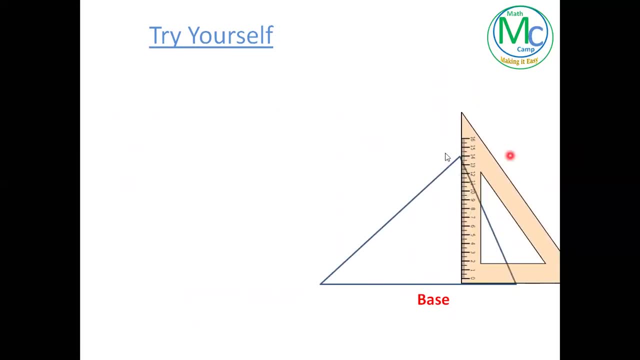 should be over the base of triangle and stop when it will touch this vertex. Draw this line And this line is going to be height For this base. Now you have another triangle. Try to find out height for this base. All right, now check your answer. So I'm going to place my set square according to the basis. 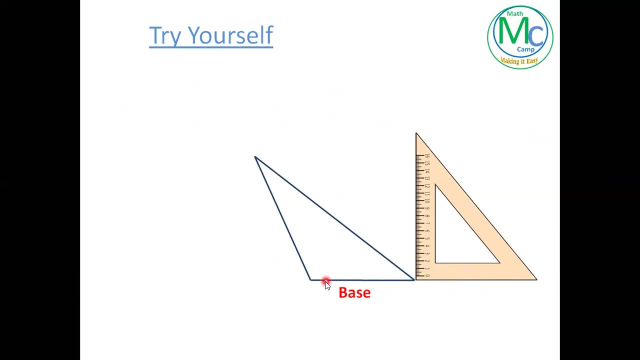 So same base base of the set square should be over the base of triangle and have an eye on this side when it will touch any of the vertex. Okay, So it is over here, All right, the height for this base is this. Now you have to check your knowledge by doing: 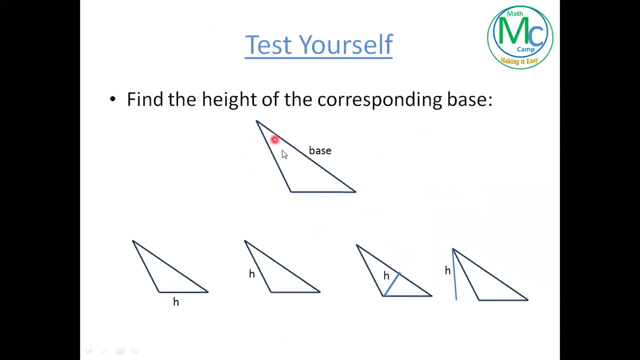 the test. So there's one question. This is a base of triangle And according to this base you have to select the height. So you have four options And all I have. they're their own heights, So you have to see which one is correct. 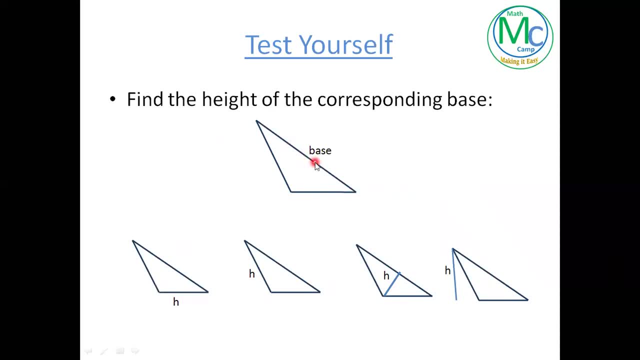 All right. So the answer for this base is this. Now I'm going to explain again this one using my set square. You can see again I'm going to place my set square. The base of set square should be on the base of triangle, Then start sliding and stop when it touch. 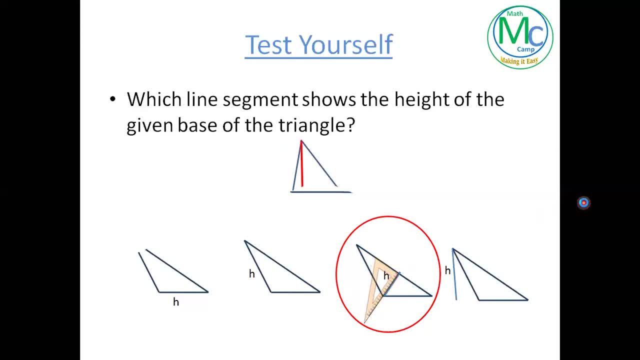 the vertex. So that means this is the height. Now you have another question. Answer this question Now. select your best option. All right, Now the height for this base is yellow line. Again, I'm going to show this one using set square, So I will place my set square the way it should be: The base of the